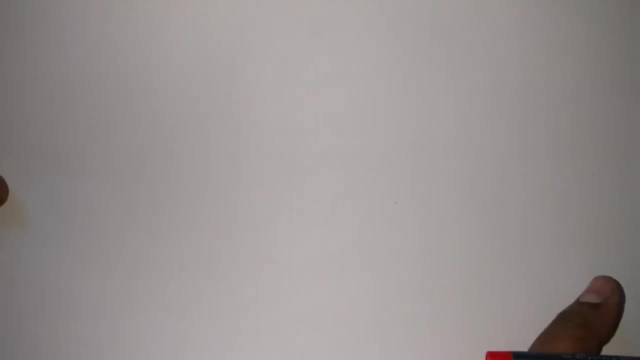 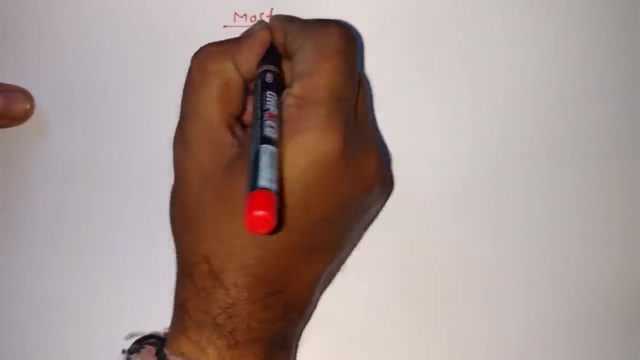 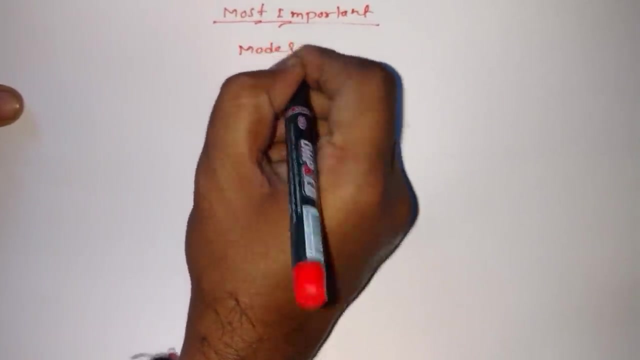 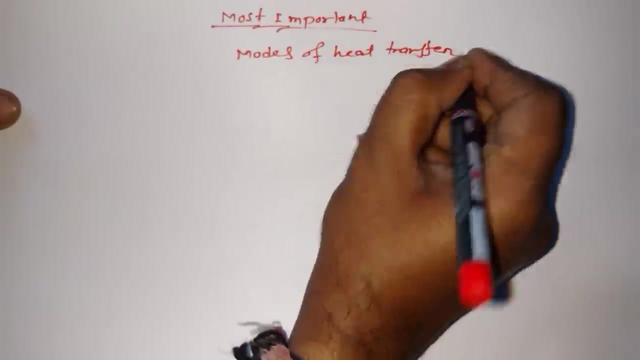 So in this video I'm going to share with you modes of heat transfer, right? so basically, I know this is not that much difficult to understand, but even then, let me share with you modes of the most important. I must say that. okay. so here the topic we are. we are considering here modes of heat transfer. so what is this? 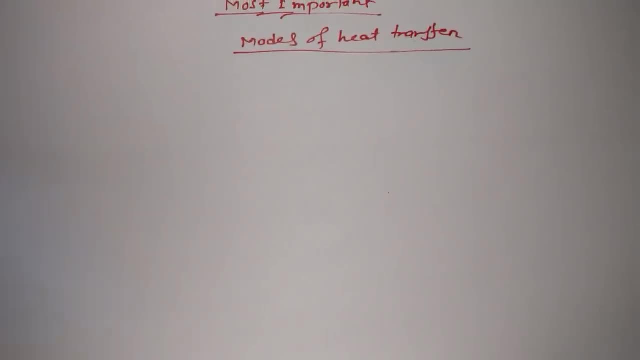 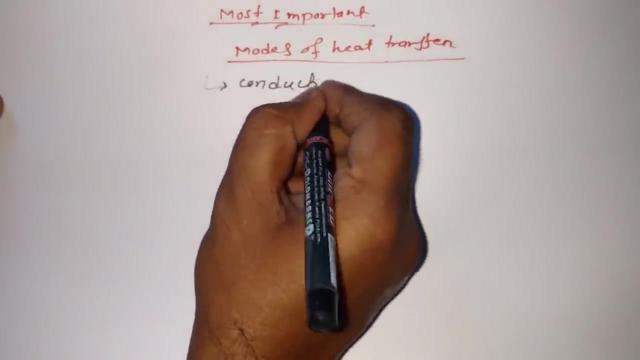 I mean modes, what? what is basically heat transfer? I have already shared with you difference between heat transfer and thermodynamics. I have already shared with you. but now modes of heat transfer. basically there are three modes, right, so let me write first. that's why you can understand also conduction, convection. 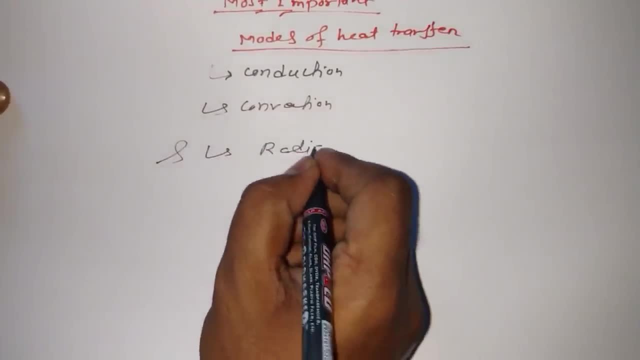 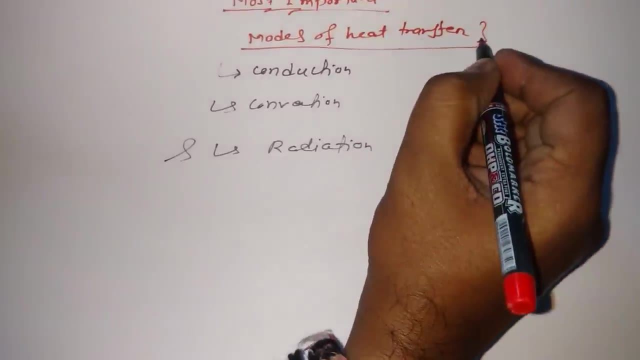 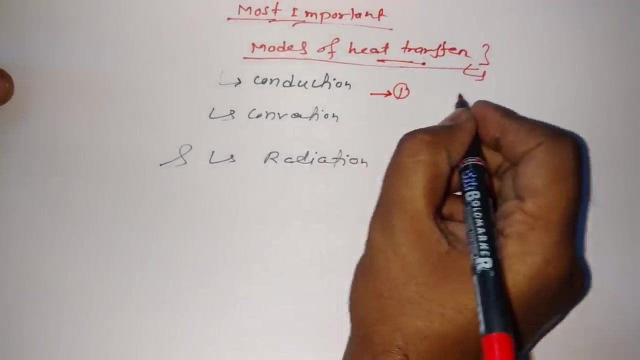 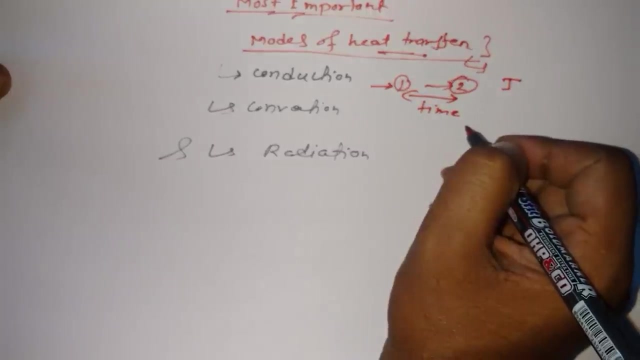 and radiation. so there are three modes of heat transfer. basically, what is here, we will, what we are going to consider here: how much heat is transferring from one place to another place, from one place to another place, with how much time? that means heat transfer, heat energy, that means the. 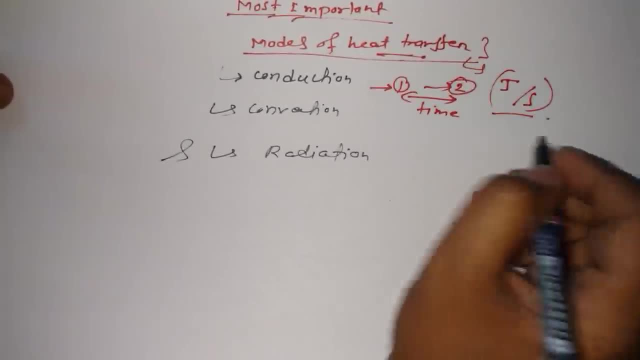 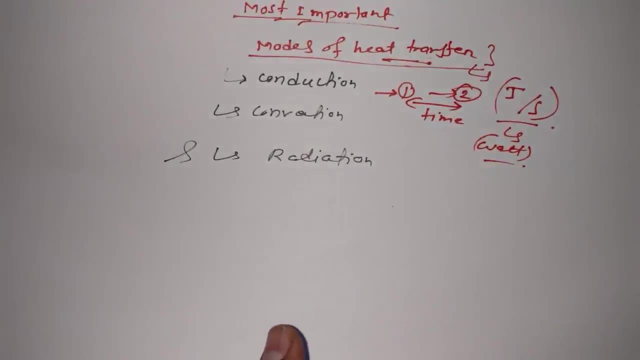 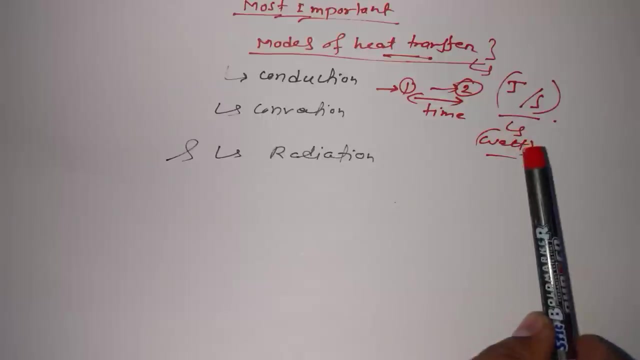 unit of energy, joule and how much time is per second. so the unit would be in watt. only one thing is pretty clear: if you are preparing for any complete examination then you have to know this: the unit of always, unit of any modes of heat transfer, would be in watt. right now, three. 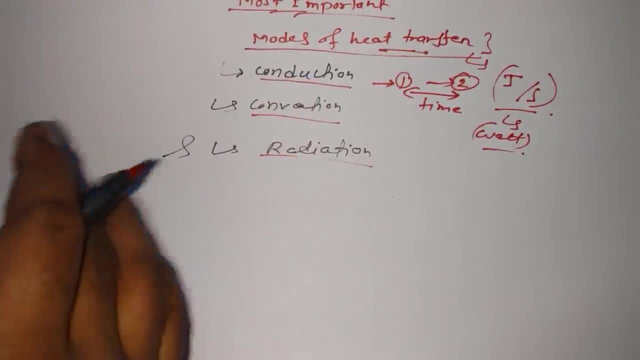 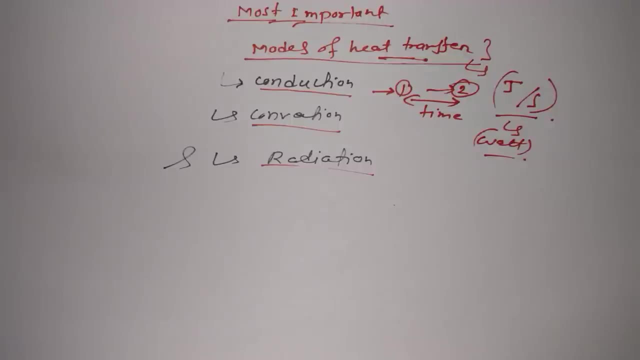 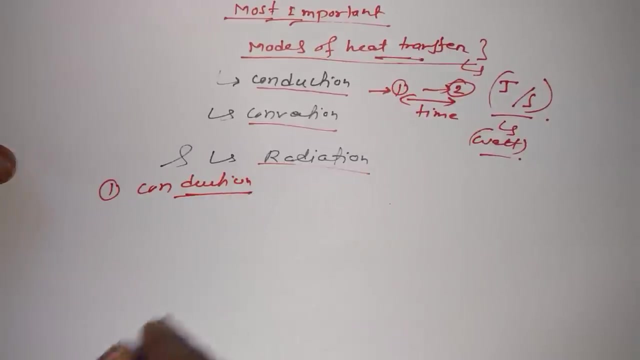 modes. let me make you understand. actually, if we'll go through in details of all these modes, it will take much more time, but today I am going to share with you some basic concept of conduction, convection and radiation. right, so let's get started with the conduction. so, basically, what is? 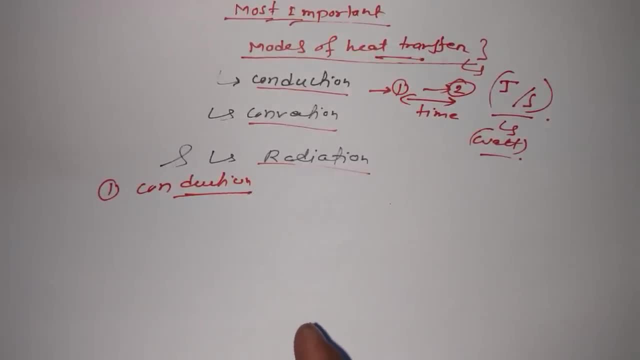 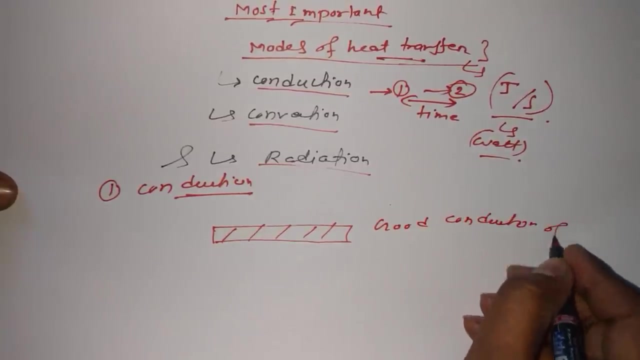 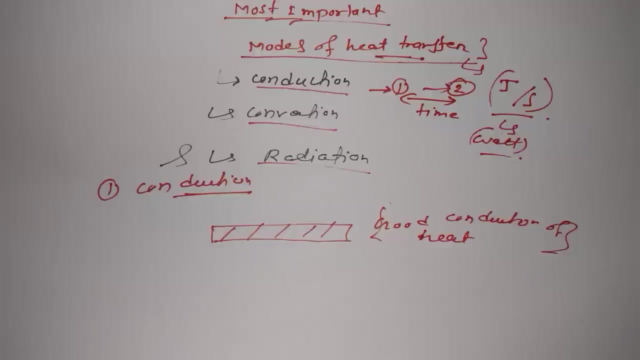 conduction. I mean generally, if heat is transferring from one place to another, in solid, not one place, I must say in solid. suppose that we have it odd metallic rod. the rod must be good conductor, good conductor of heat or electricity, because in general, if any metal or any of any, anything is good, 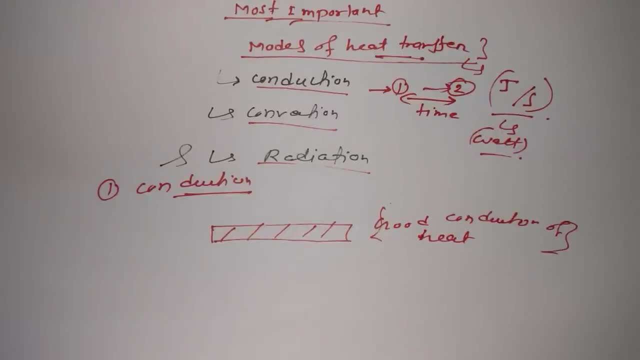 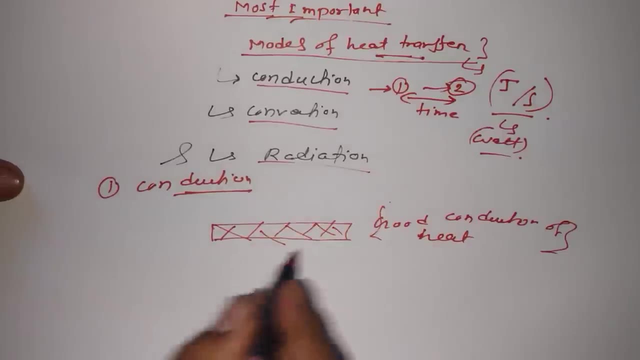 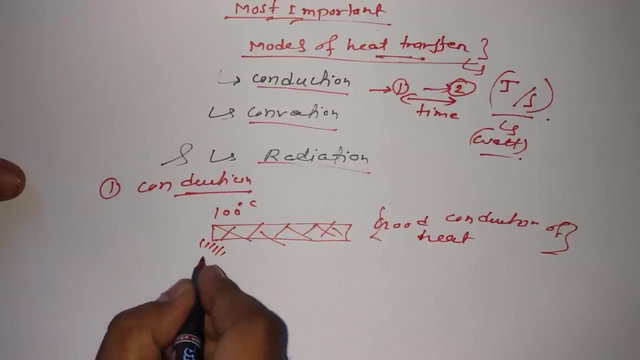 conductor of electricity, that thing is also good conductor of heat. this is in general. this is a simple concept. right, white is happening. mixture with you, right? so what is conduction if temperature is 100 degree here? and I am providing sources through a lamp, suppose that, and lamp is. 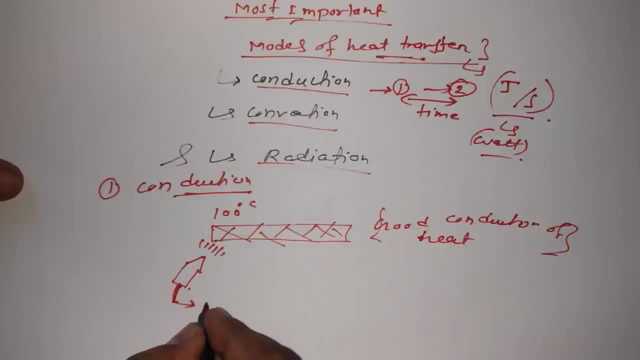 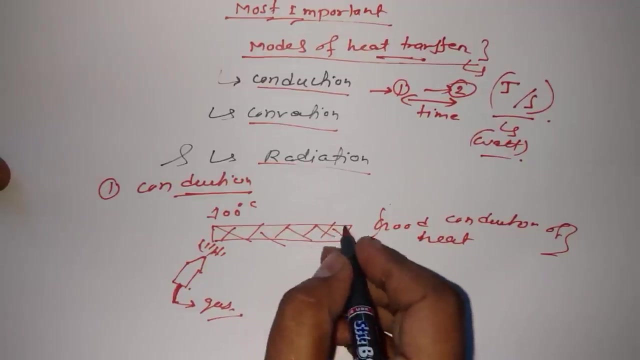 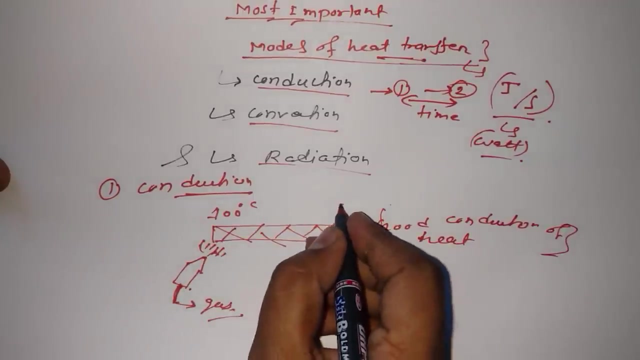 connected with some, you know some, maybe gas. right, we are sources providing sources for temperature, and here the temperature is 100 degree centigrade and as well, as usual, that we are not providing any source of heating here. so that means the temperature would be less than less here than here. so let's say: 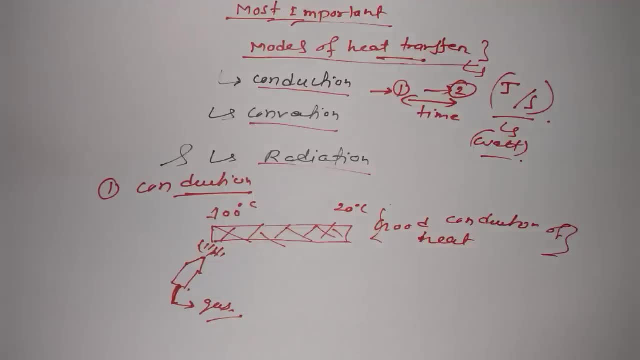 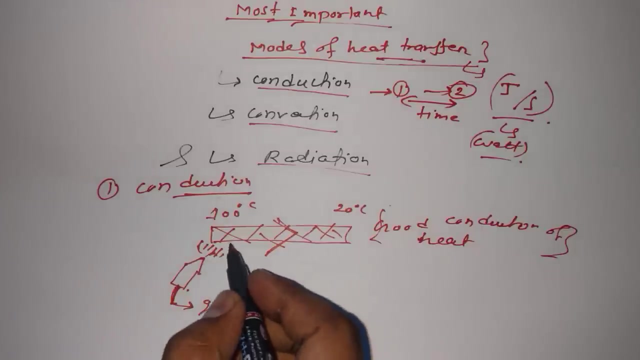 the temperature is here, right? so in this process, what will happen? the temperature will flow. the direction would be like this: because temperature is always flow from, I mean heat is always flow from higher temperature to lower temperature. that is why it is happening, right? so why it is happening when, why the heat is. 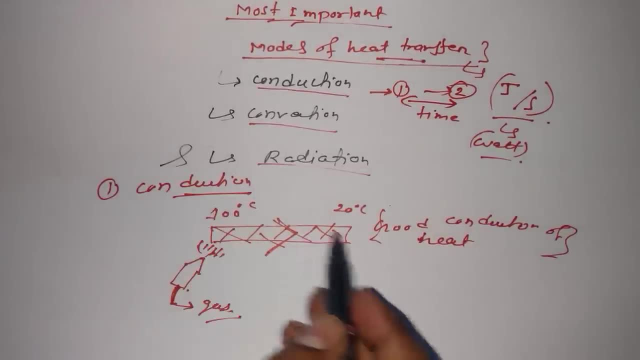 flowing from here to here. why not from here to here? okay, so this is the concept, right, because you know, here, 100 degree centigrade we are having, here, we had having to, 180 degree centigrade, white is flowing from here to here. that is the you know, that is the universal truth, that heat always flow. 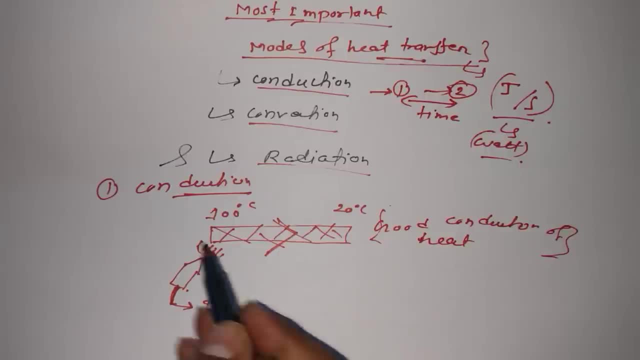 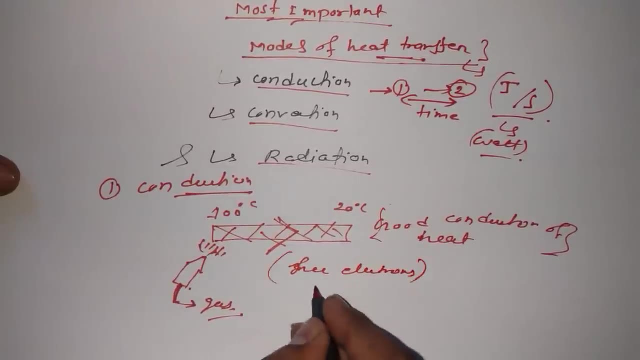 from higher temperature to lower temperature, but white is happening. that's because of free electrons. there is about 70% percent reason behind is: this is happening because of electrons present in this metal, and this is a good conductor of electricity. that's because of also, that's because of also free electrons, right? so, uh, that that's because of electrons, not only the one. 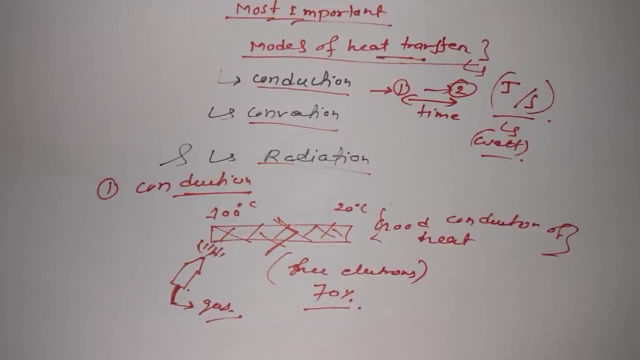 reason. there is another, another few reasons, just like because of lattice vibration. also, in solid, heat transfer is taking place because of lattice vibration, but most of the, the main reason is free electrons, right? so this is happening in solid. so most of the time conduction happen in solid. but 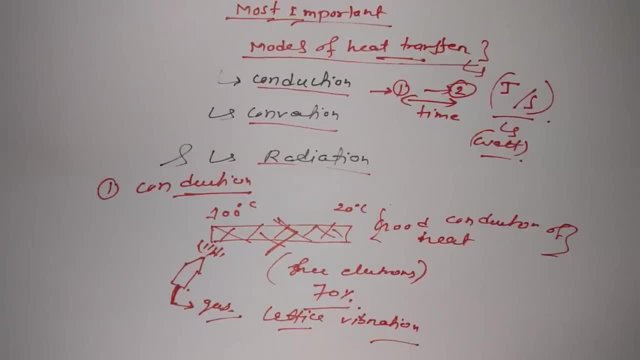 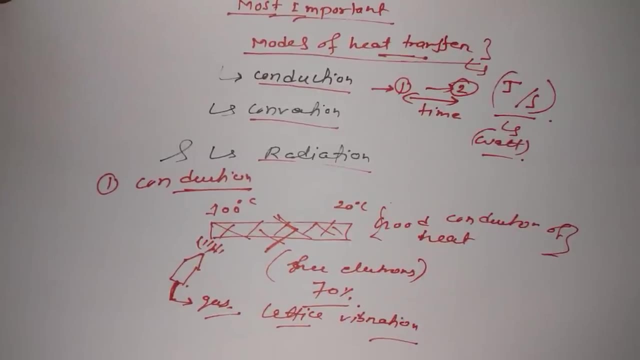 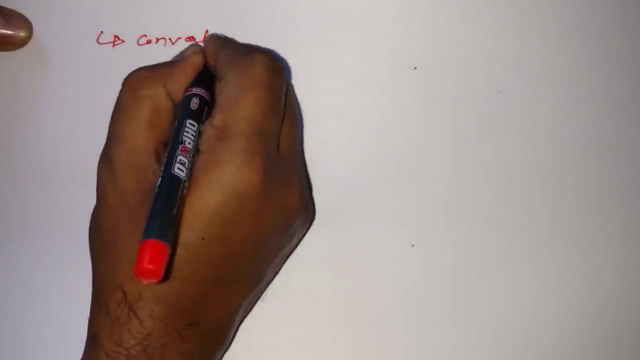 it can be happen also in liquid. it can be happen also in gas. you need to consider all these three, right? so let's go for another mode of heat transfer. that is convection. right, okay, let's go for it- convection. so what is convection? basically, let me write: convection- what? 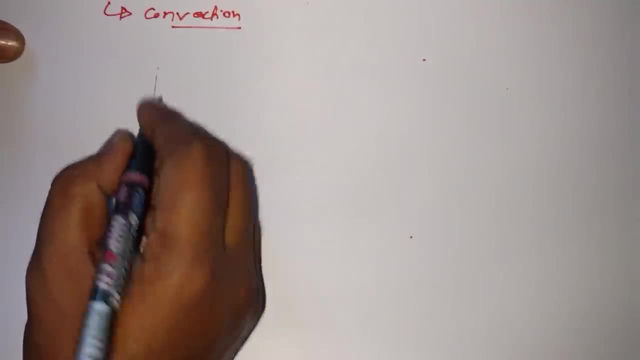 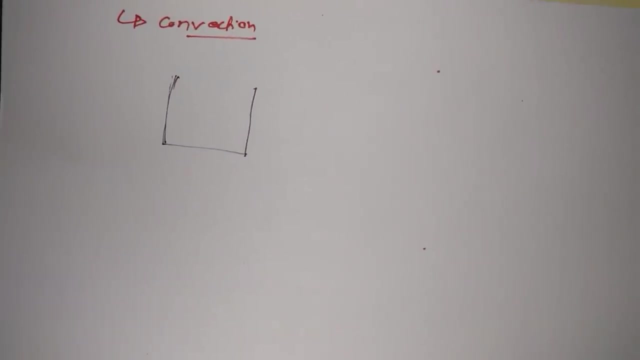 is convection, basically. uh, suppose that you know? we all know the winter season is going on, right? i don't know when you are watching this video, but let me share with you as i am making. i am creating this video in the winter season. so if this is just november, about november, okay. 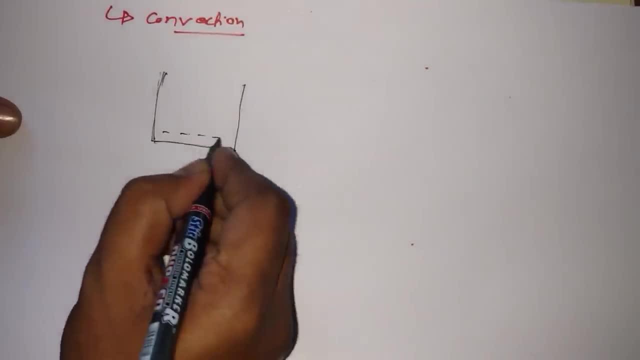 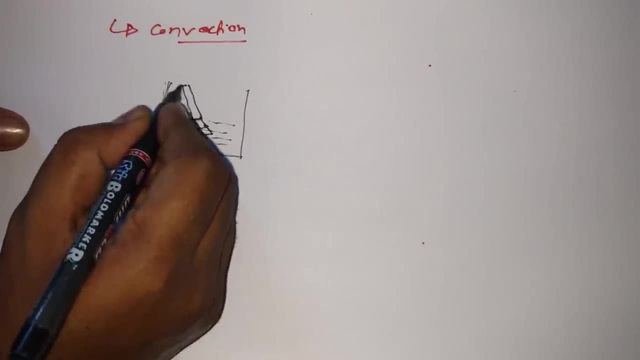 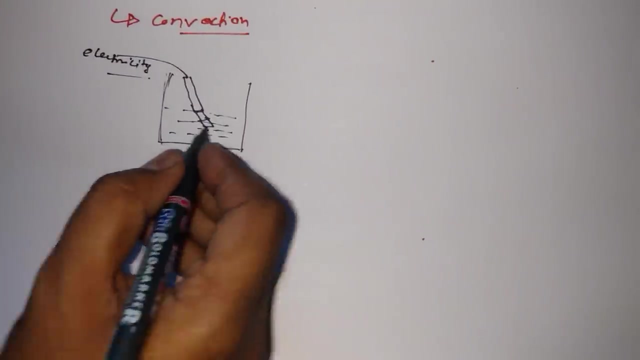 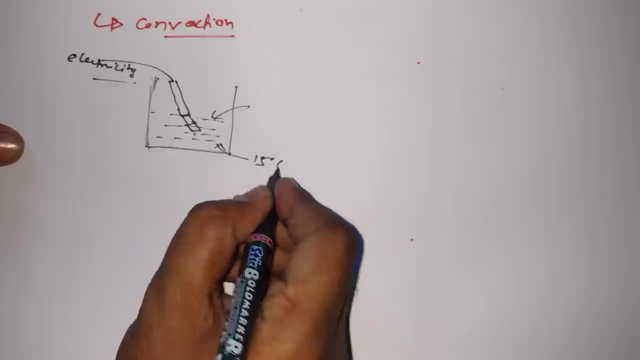 so winter season is going on. so what we do exactly? we're having water here, okay, so we are putting, suppose that rod. rod we are putting, and rod is connected to it, electricity, electricity, right, and what will happen? you know after few minutes that if the temperature is right now, suppose that 15 degrees centigrade, after a few minutes temperature would 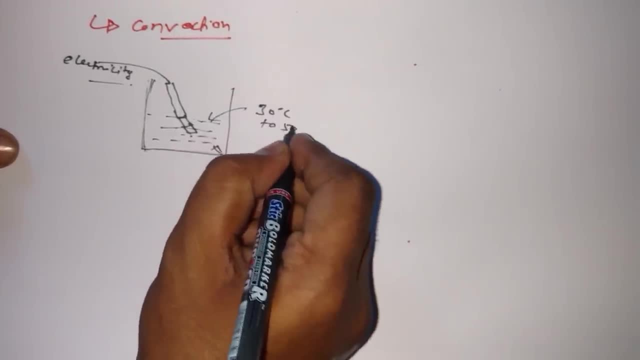 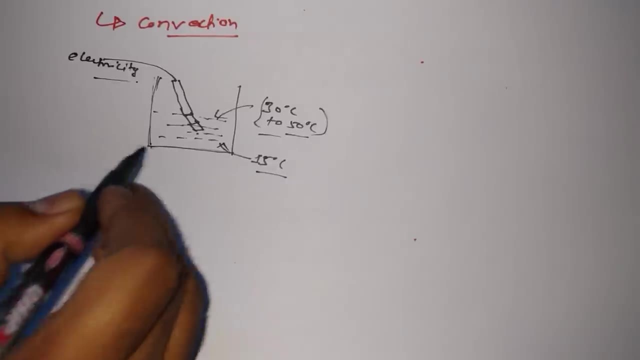 be around 30 degrees centigrade, or even 50 degrees centigrade, okay, and after, if we'll, if i'll keep on, keep putting this rod inside the water, then temperature will be increased to about 70 degrees centigrade. maybe 100 degrees centigrade then again. 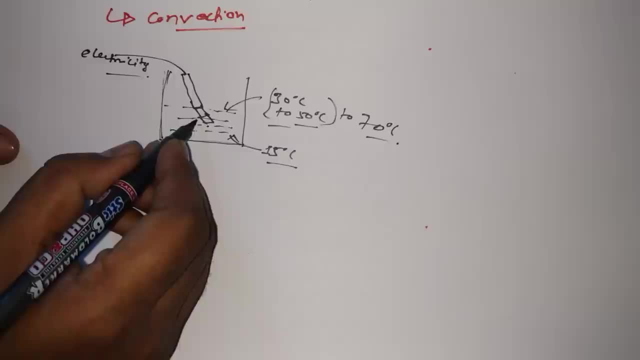 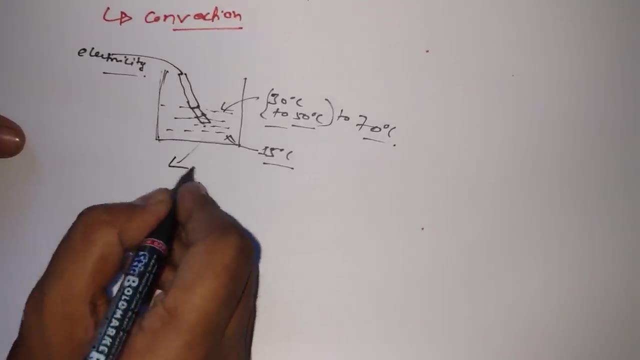 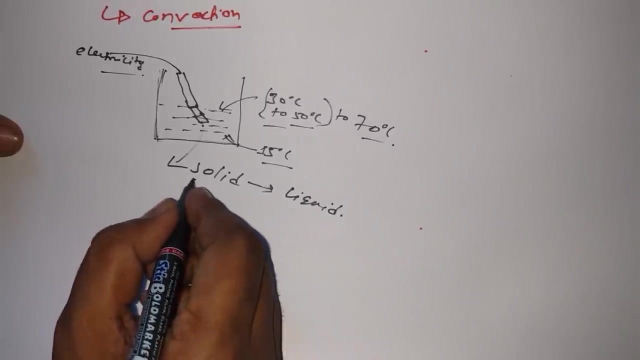 it will be keep on increasing because you know we are supplying heat inside the temperature, inside the water. that means what is happening here: from solid, the rod is in solid and it is going to a liquid. heat is transferring to liquid. that means from: if heat is transferring from solid to liquid. 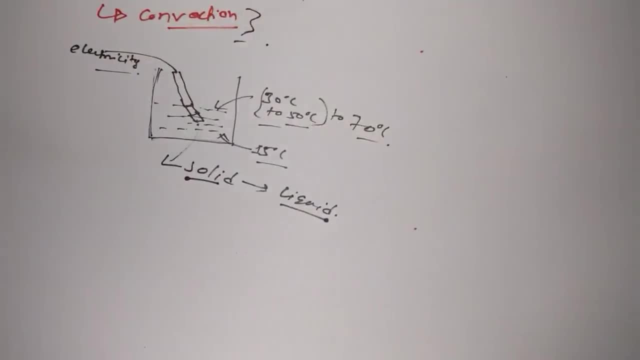 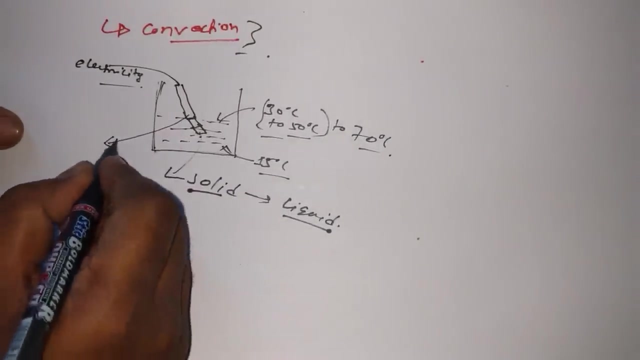 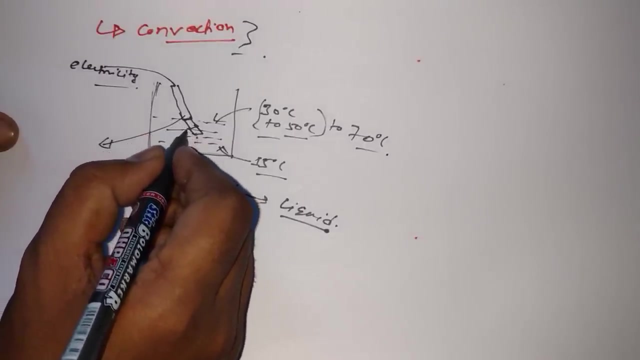 then that process is known as convection because of convection process. that is, uh, that is happening. i must say that, okay, because of convection process. only now the thing is that white is also happening. simple, if we are put, we are, we are supplying electricity. okay, that means what is happening here, the rod or 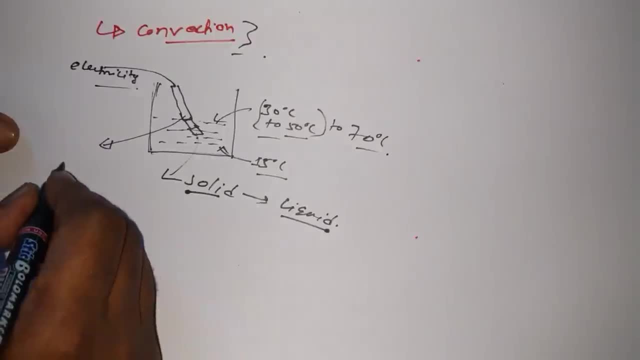 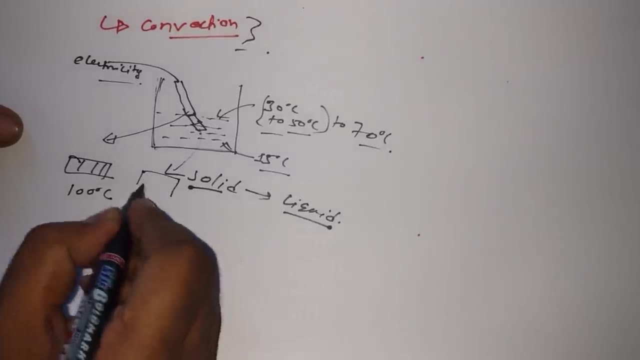 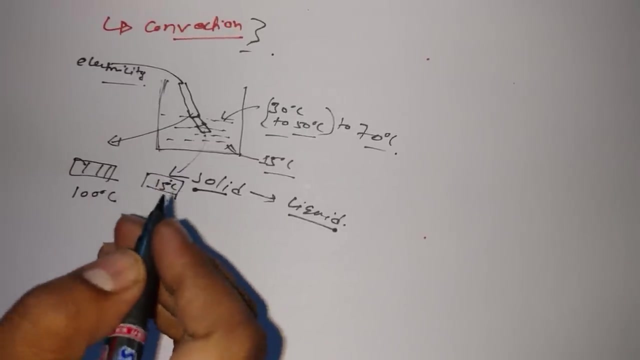 temperature of rod is increasing, keep on increasing. so if the rod temperature is 100 degrees centigrade- suppose that- and water temperature is only 15 degrees centigrade, then according to universal law, what? what is happened with the heat? heat always flow from, always flow from higher temperature. 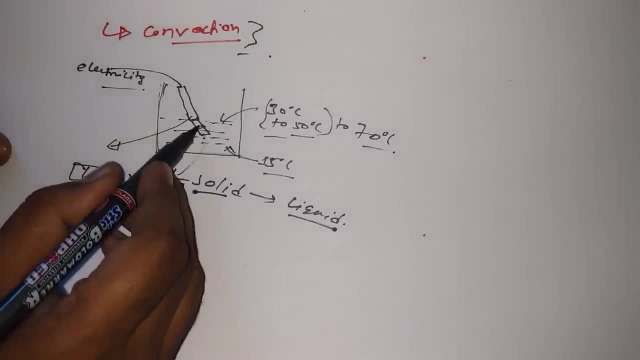 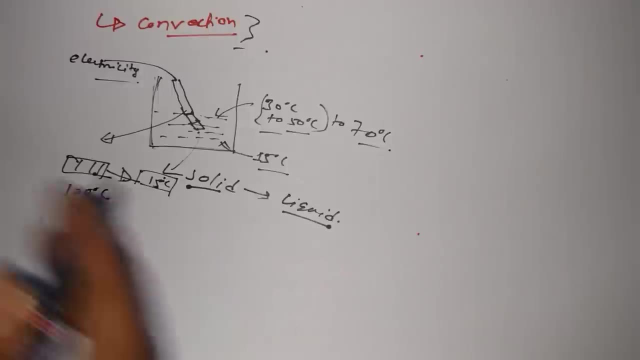 to lower temperature. that's why the temp, the heat, is flowing from broad to water and that is the reason the temperature of water is keep on increasing. so this is the process. i mean this. is it about convection? now we have a lot of things to study in convection, just like newton's law. 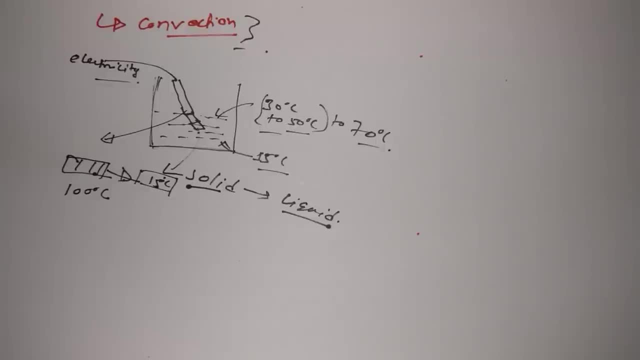 and there are many uh dimensionless number are there, so let me explain how to study convection. and there are many uh dimensionless number are there, so let me explain how to study convection there. so we will. we will go through all those dimensionless number. that's why you will understand. 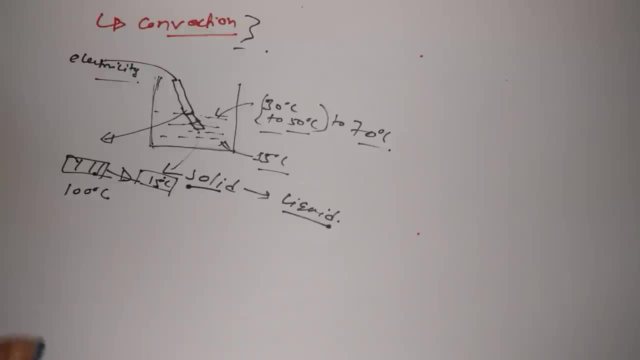 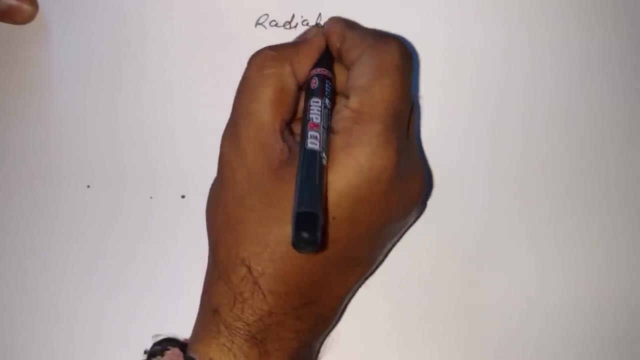 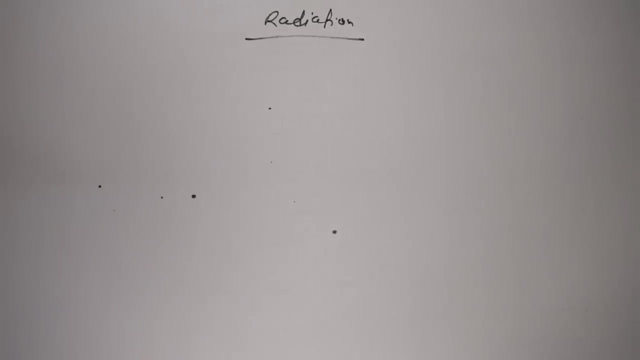 each and everything about convection, right, so this is all about convection. so one last is remaining, that is radiation, radiation. so, uh, this is also, you know, this is a radiation process we are now utilizing because it's a i have already shared with you. it's a winter season, right? so what we? 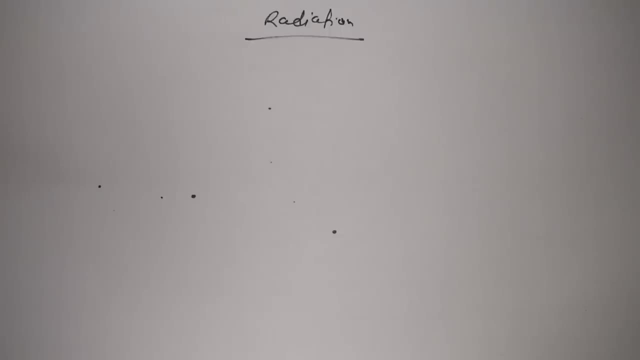 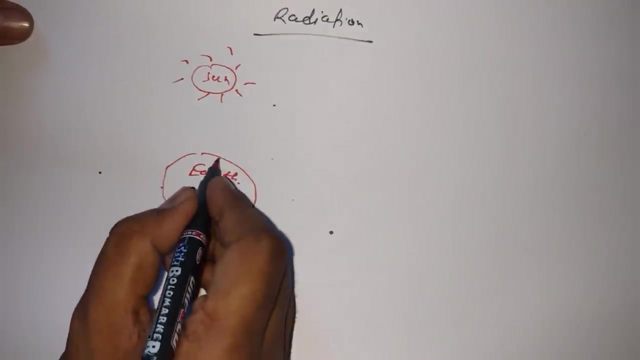 usually do we go outside and get some vitamin d because from sun, right, so suppose that this is sun and this is earth in general, earth is smaller than sun. okay, but even then i let me share with you, so as i am sharing with you, that i am look, i am on the earth and i am looking at the sun. so suppose 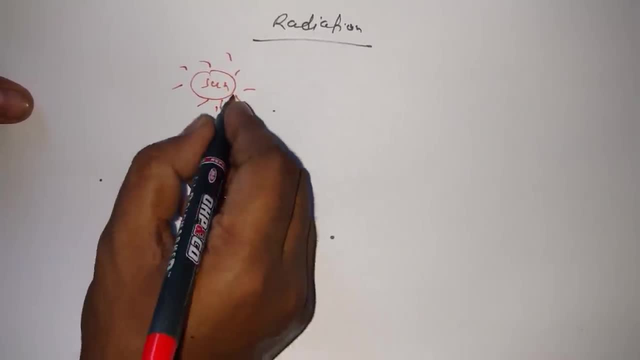 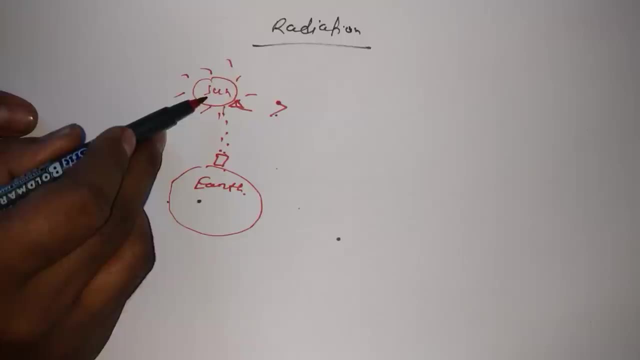 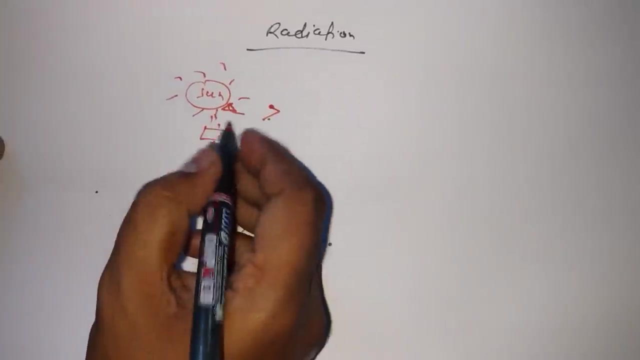 that you are here and what is happening? what is happening? the temperature of sun is much more than earth. that is truth. that's why heat is flowing from sun to earth. but is there any medium between this? you or i must say: earth and sun, no, no, there is no physical medium. there is no physical 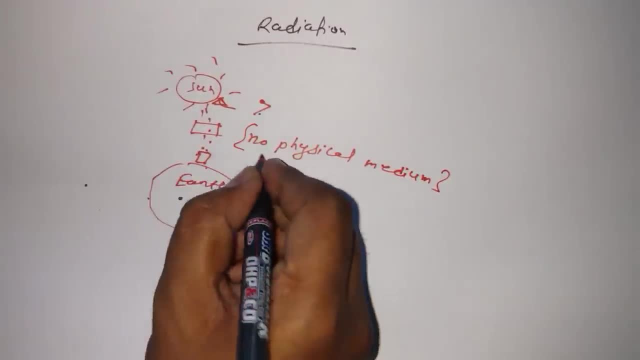 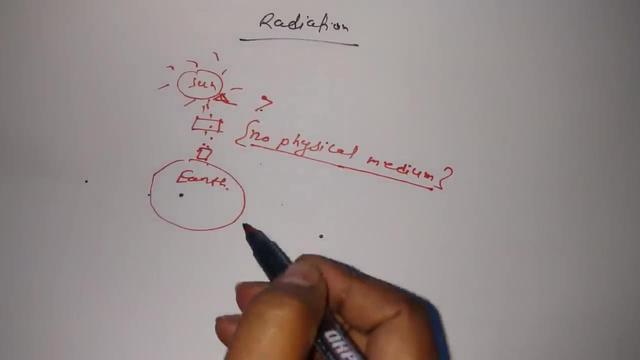 medium and what i have shared with you just right now. this sentence is most important in case of radiation. yes, now look at this. i mean, if there is no physical medium in between source, you can write that this is sun. this sun is going to be in between the earth and the sun. 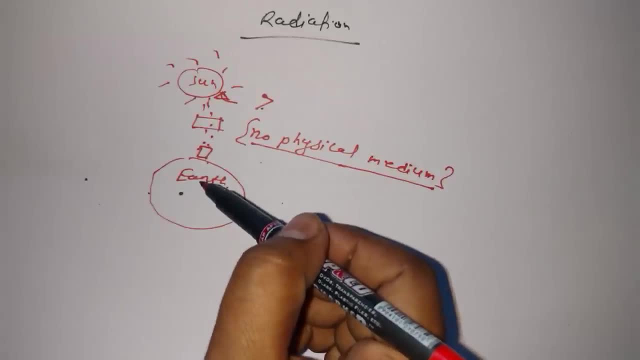 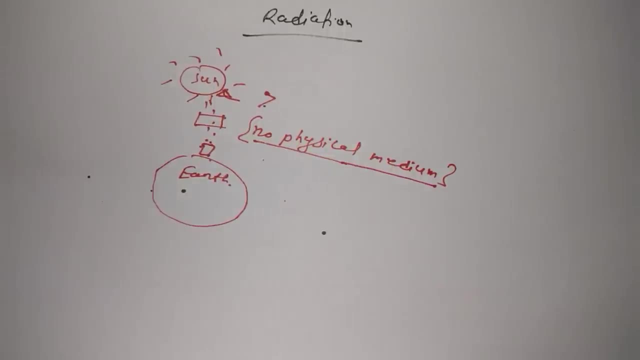 between the earth and the sun, because if there is no physical medium in between the earth and sun, in between the source and the person is taking or utilizing that heat, then that process is known as radiation. there should not be any physical medium. so you need to remember this sentence. 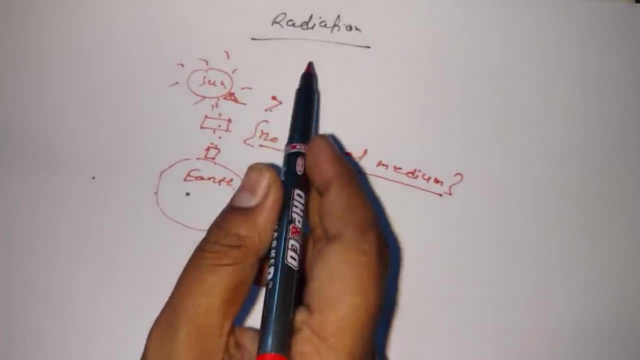 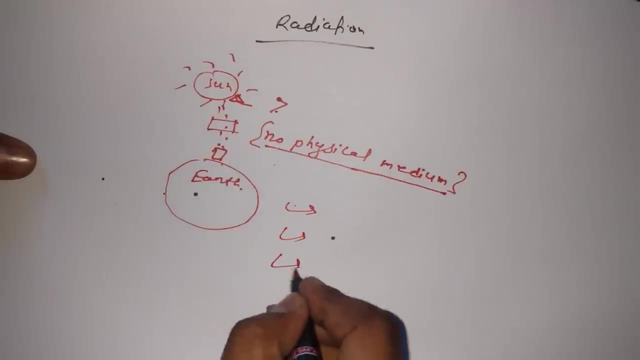 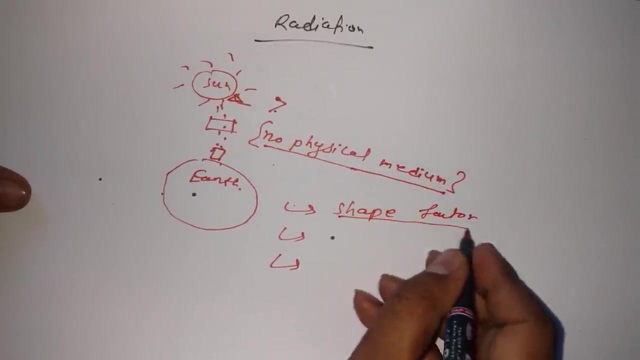 because this is the most important sentence in this process. in radiation we are having lot of laws and most important factors let me share with you. if you are preparing for gate, then we need to understand shape factor. i have already shared with you a few numerical- previous and numerical. 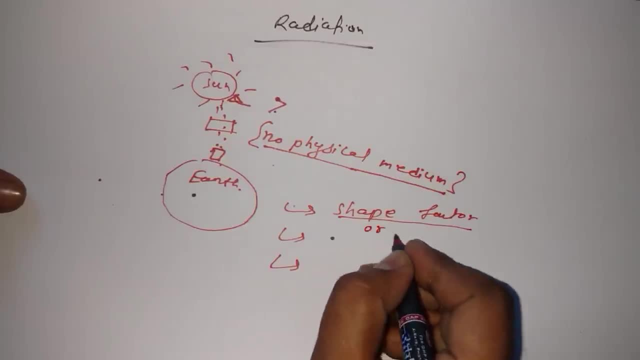 problems of gate related to shape factor, or there is another name of this, that is view factor. there is one of the uh. one of them must say law is there or theorem is there? that is a reciprocity theorem that is important in shape factor to solve the numerical problems with 100. 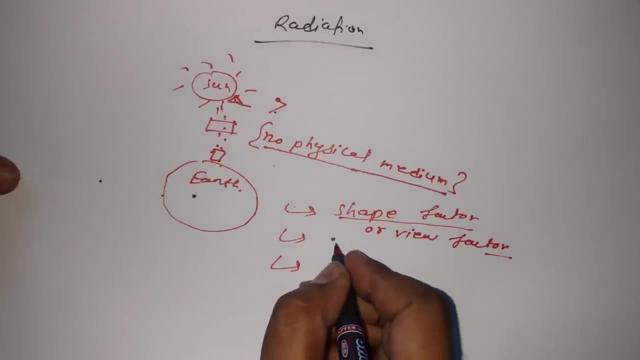 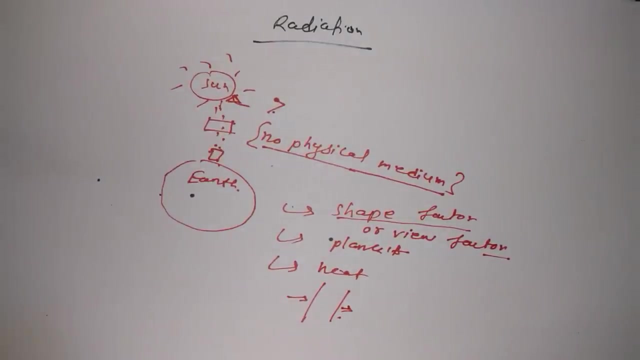 almost 100 accuracy. now, another thing is that uh, planks constant and, and you know, heat transfer taking place between two rods, parallel rods, or maybe you know infinite rods, so that is also important. so there, you need to understand stephen bolchman law, stephen. 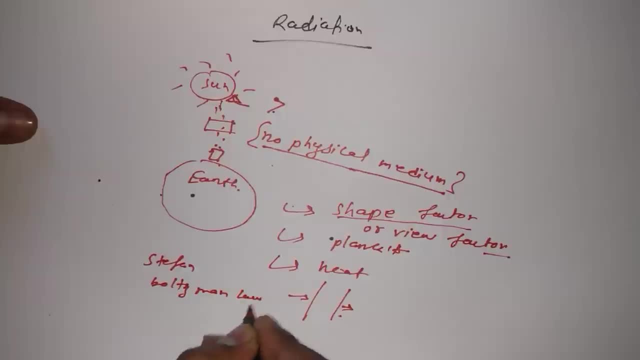 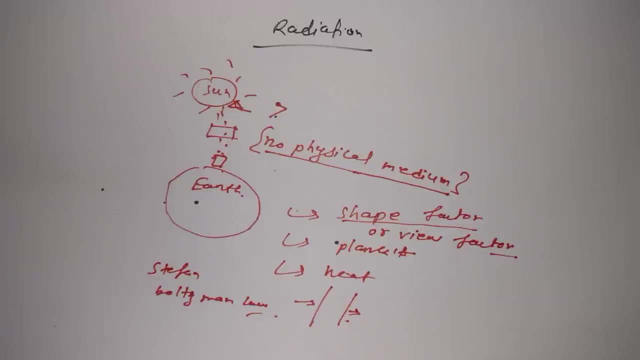 bolchman law. so you need to, you need to understand this law also in if you are preparing for computer examination, if you are preparing for university examination, then you need to go through all things and you need to actually have at least a overview of all- uh, all topics, all topics. that's why you cannot write, at least in the university. 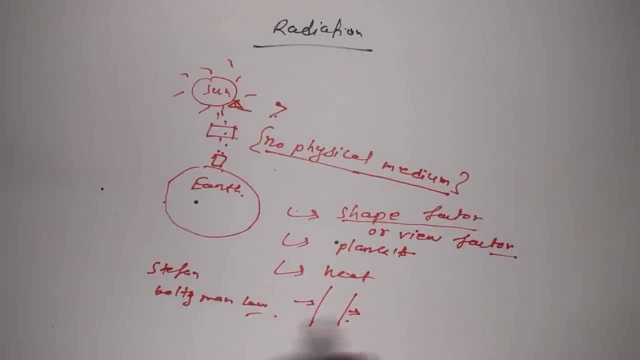 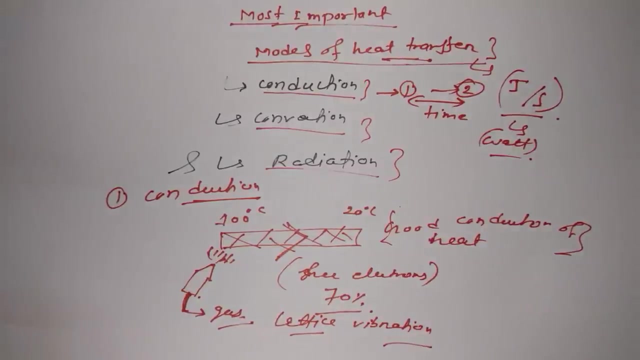 examination, right, so so what i was thinking, i was talking about like this. so, basically, what is happening here? what is happening here, all these processes in all these processes- i mean all these processes means these processes- conduction, convection and radiation- we need to understand one thing: that is happening, what is happening, all these processes, that is. 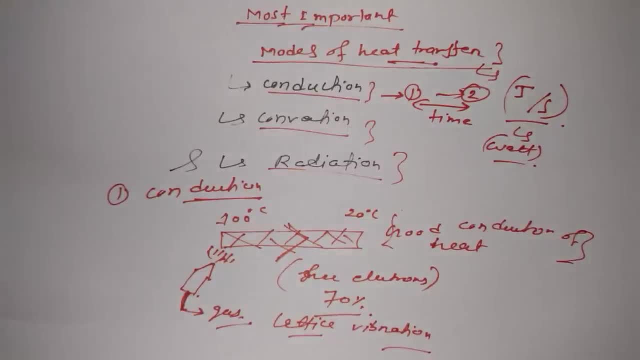 joule per second. i mean energy. heat energy is transferring from one place to another place with respect to time. we are considering that that is most important to remember and go for it. so we will understand all these things in details in my next videos. thanks for watching. see you soon in my next video. bye, bye.